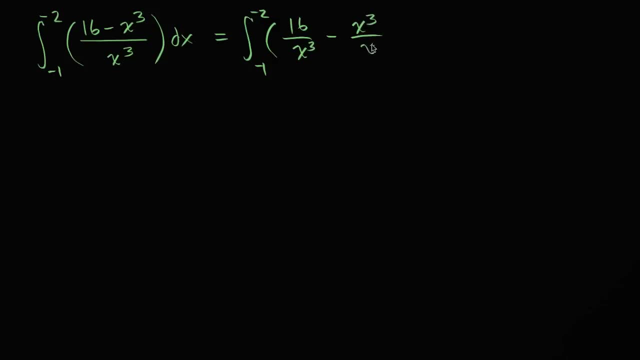 minus x to the third, over x to the third, Minus x to the third, over x to the third, dx. And now, what is that going to be equal to? That is going to be equal to the definite integral from negative one to negative two of: 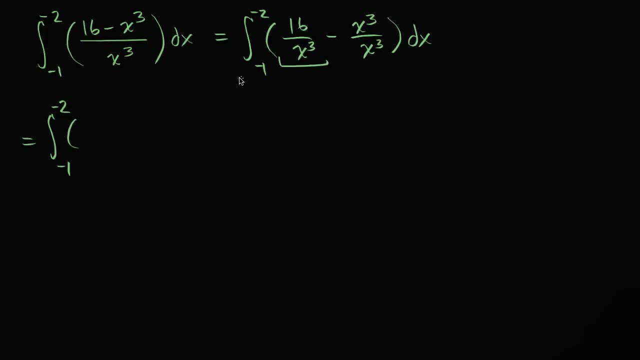 I could write this first term right over here. Let me do this in a different color. I could write. I could write this As: 16: x to the negative, three, x to the negative three And this second one we have minus x to the third. 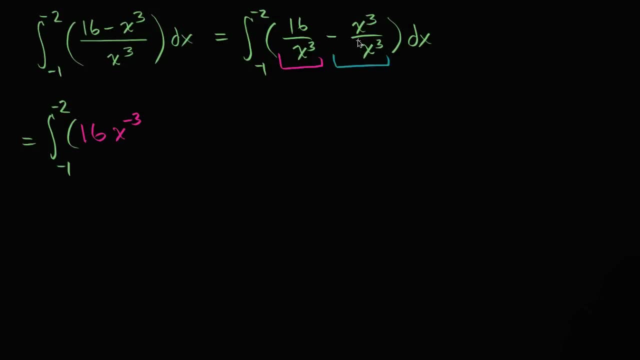 over x to the third. well, x to the third is just over x to the third. over x to the third is just going to be equal to one. So this is going to be minus one dx, so dx, And so what is this going to be equal to? 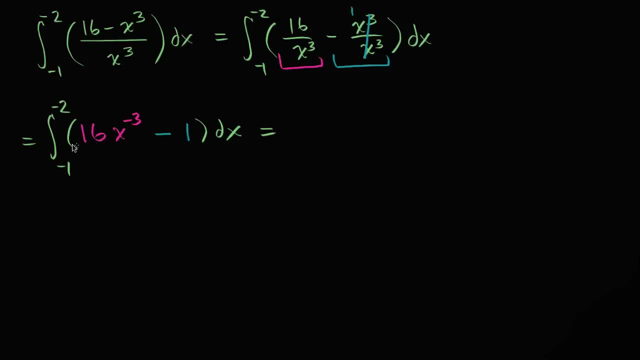 Well, let's take the antiderivative of each of these parts, and then we're going to have to evaluate them at the different bounds. So let's see the antiderivative of 16 x to the negative three. We're just going to do the power rule. 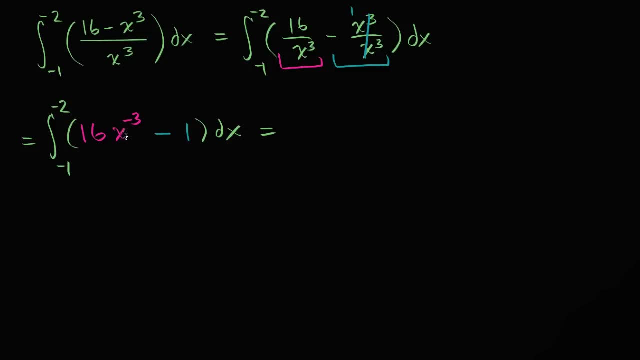 for derivatives. in reverse, You could view this as the power rule of integration for, or power rule of taking the antiderivative, Where what you do is you're going to increase our exponent by one, So you're going to go from negative three to negative two. 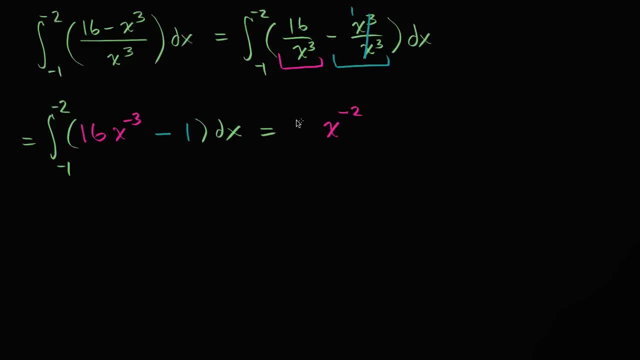 And then you're going to divide by that amount, by negative two. So it's going to be 16 divided by two. So it's going to be 16 divided by two, So it's going to be 16 divided by two. 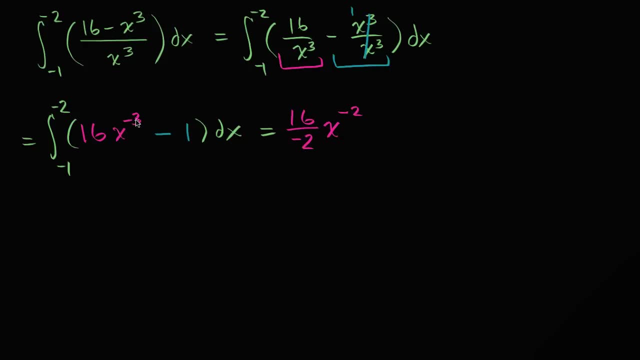 16 divided by negative, two times x to the negative two. All I did is I increased the exponent and I divided by that amount. So that's the antiderivative here. And 16 divided by negative two, that is just negative eight. 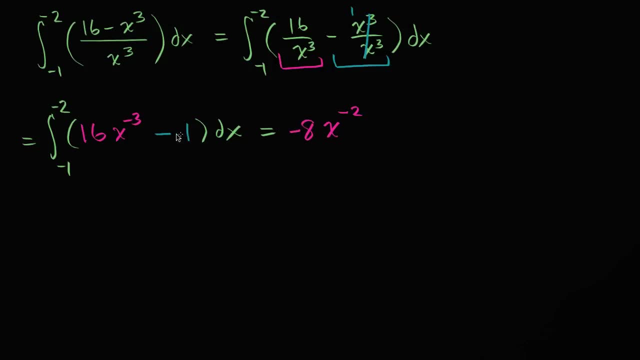 So we have negative eight, x to the negative two, And then the antiderivative of negative one. well, that's just negative x, Negative, negative x, Negative x. And actually you could, you might just know that. And then, hey, if I take the derivative, 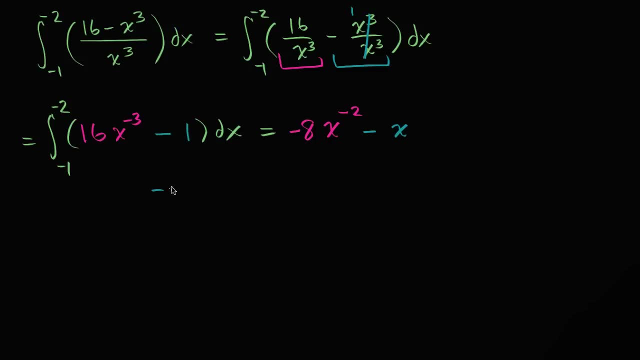 of negative x, I get negative one. Or if you viewed this as negative x to the zero power, because that's what one is, well, it's the same thing. You increase the exponent by one to get x to the first power. 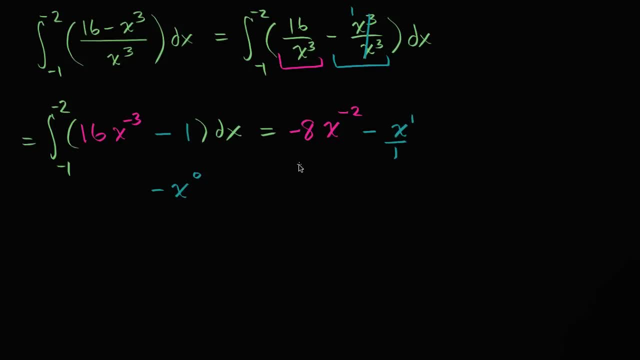 And then you divide by one, And so, yeah, I mean you could view it as that right over there, But either way you get two negative or minus x. And so now we want to evaluate that. We're going to evaluate that at the bounds. 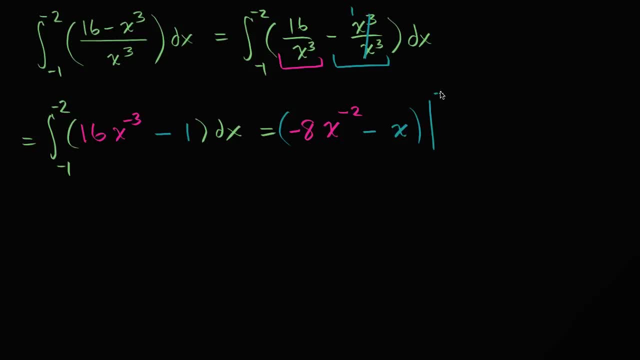 and take the difference. So we're going to evaluate that at negative two And then subtract from that this evaluated at negative one, And let me do those in two different colors, just so we can see what's going on. So we're going to evaluate it at negative two. 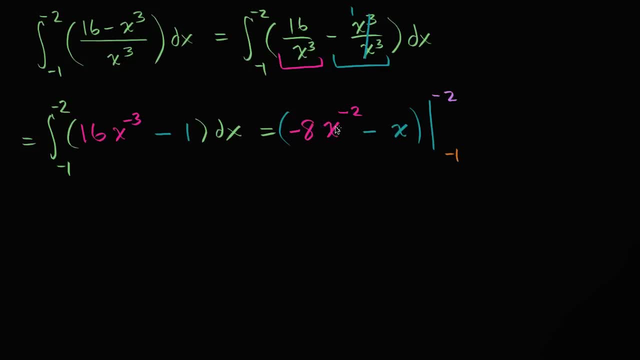 And we're going to evaluate it at negative one. So let's first evaluate it at negative two. So this is going to be equal to. this is going to be equal to when you evaluate it at negative two. it's going to be negative eight. 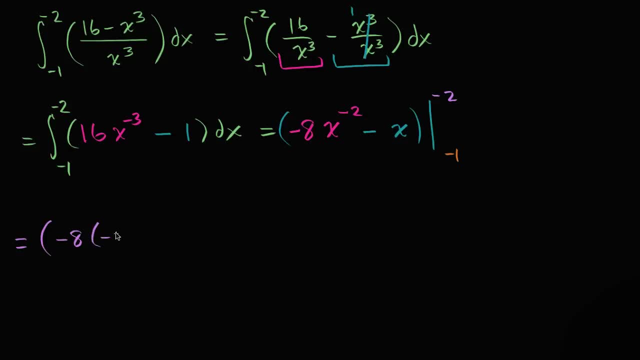 negative eight times x to the negative two. So negative two to the negative two, negative two power minus negative two. And from that we're going to subtract it, evaluate it at negative one, So it's going to be negative eight times negative one to the negative two power. 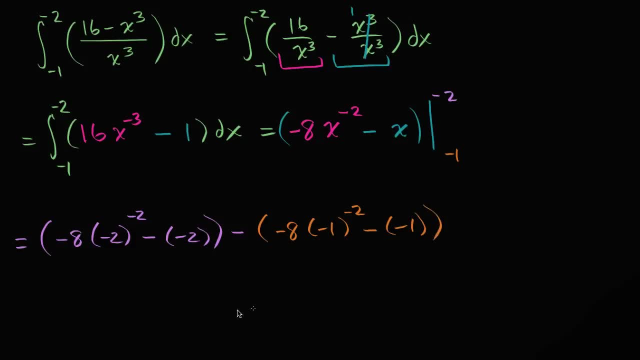 minus negative one. All right, so what is this going to be? So negative two to the negative two. so negative two to the negative two is equal to one over negative two squared, which is equal to one-fourth. So this is equal to positive one-fourth. 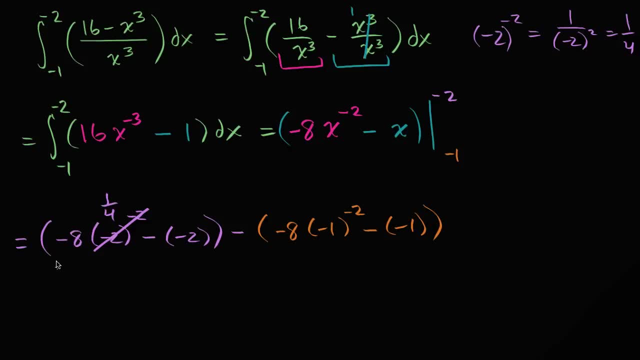 But then negative eight times positive. one-fourth is going to be equal to negative two, And then we have negative two minus negative two, So that's negative two plus two, And so everything I've just done in this purplish color, that is just going to be zero. 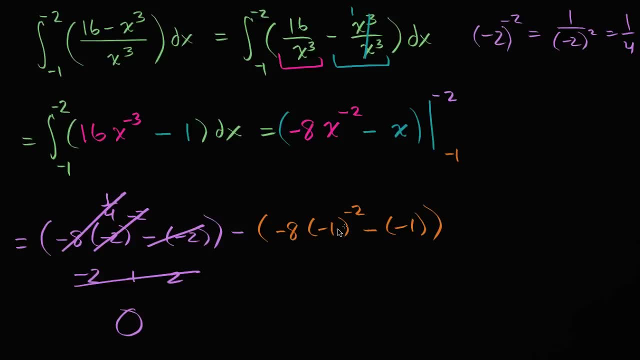 And then, if we look at what's going on in the orange, when we evaluated negative one, let's see negative one to the negative two power. well, that's one over negative one squared. Well, this is all just going to be one. 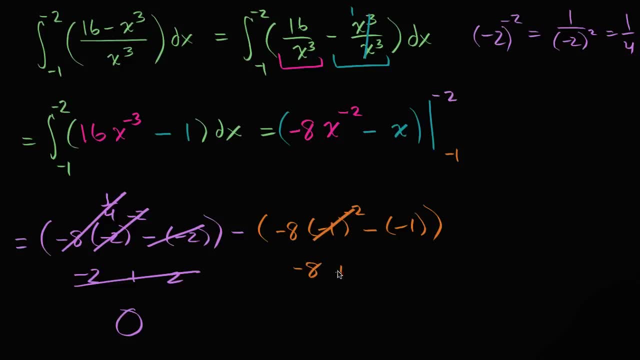 And so we're going to have negative eight plus one, which is equal to negative seven. So all of this evaluates to negative seven, But remember, we're subtracting negative seven, And so this is going to result. we deserve a little bit of a drum roll.